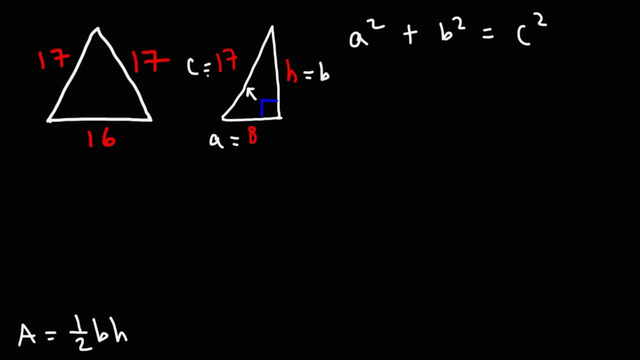 The hypotenuse, which is across the right angle. That's c. That's going to be the longest side of the triangle, which is 17. So, now let's plug in what we have. 8 squared plus b is going to be h. So, this is h squared. And c is 17. 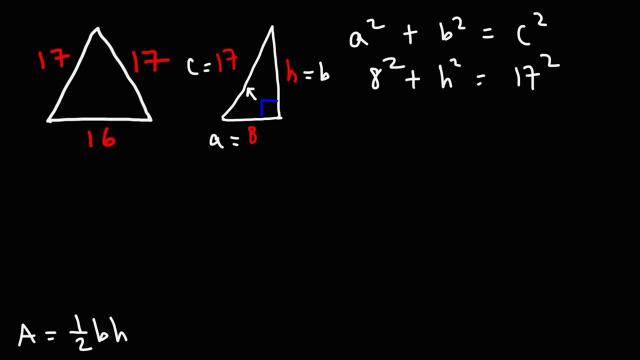 Now, 8 squared. 8 squared is 8 times 8, which is 64. 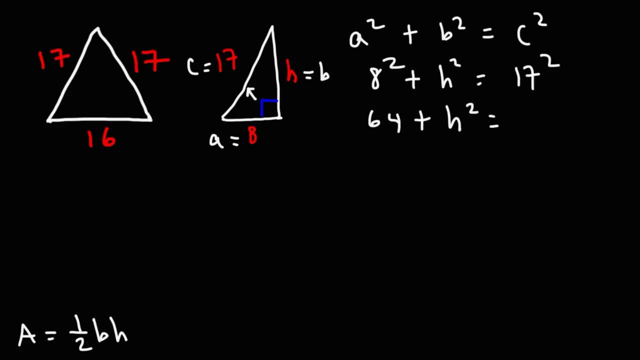 17 squared. I'm going to have to use a calculator for that. 17 times 17 is 289. 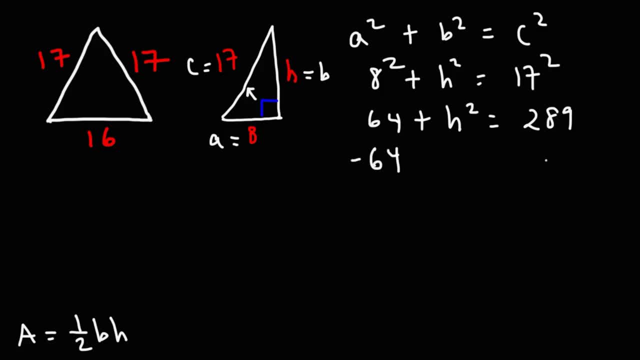 Now, to get h squared by itself, we need to subtract both sides by 64. And we can bring down the h squared. So, 289 minus 64 is 225. Now, to get h by itself, we can take the square root of both sides. 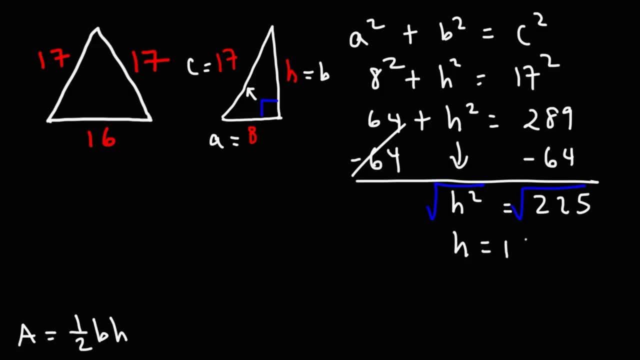 And the square root of 225 is 15. So, the height of the triangle is 15 units. 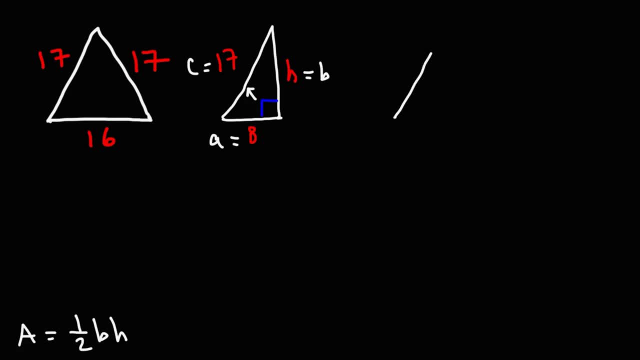 Now, let's redraw the original triangle. But only with the relevant parts that we need. So, the base is still 16. But the height, we know the height to be 15. 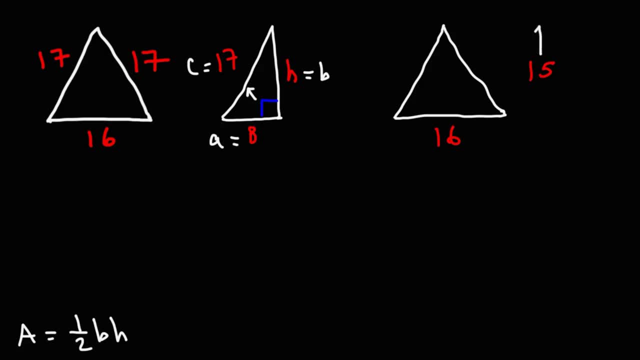 So, this is the 8, 15, 17 triangle. So, now we can calculate the area. Now that we know the values of b and h. 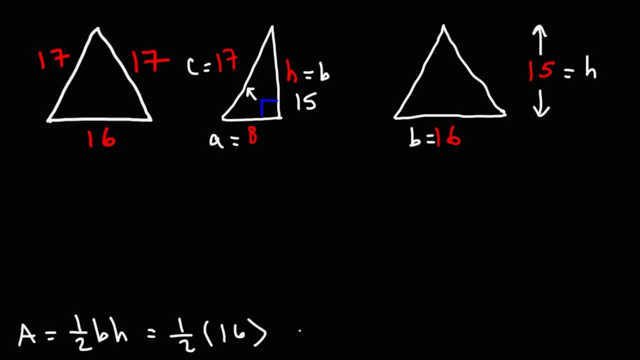 So, it's 1 half times the base, which is 16, times the height, which is 15. Half of 16 is 8. And 8 times 15 is 16. And 8 times 15 is 16. And 8 times 15 is 16. 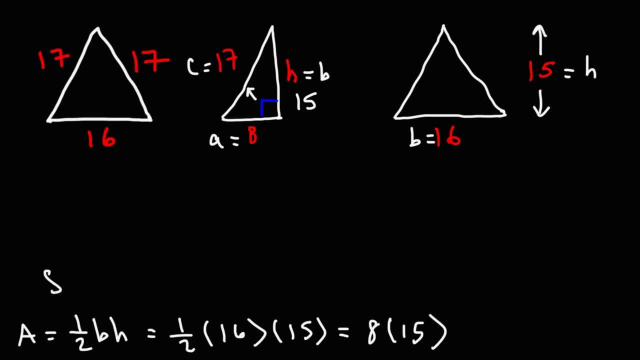 If you want to do it mentally, you can write it this way. 15 is 10 plus 5. 8 times 10 is 80. 8 times 5 is 40. 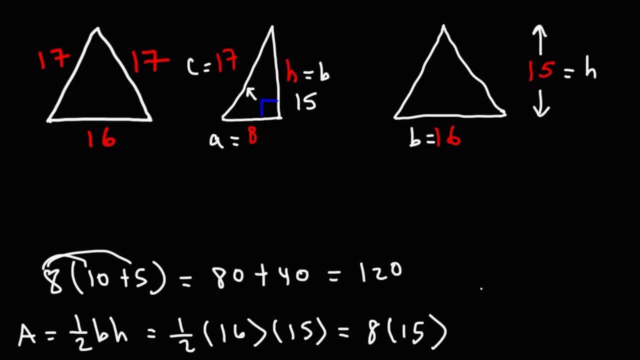 So, this is going to give us 120. So, that is the area of this particular isosceles triangle. It's 120 square units. 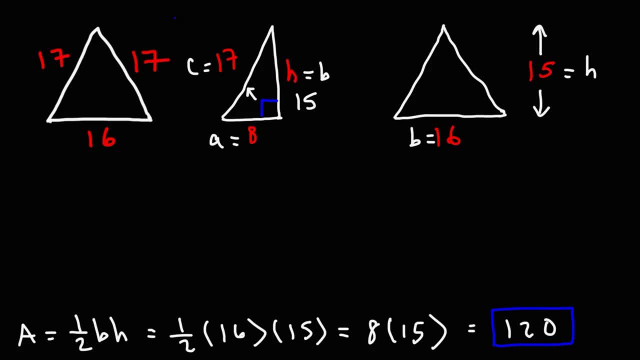 Now, let's talk about another way in which we can get the answer. Anytime you know all three sides of a triangle, you could use Huron's formula. And here it is. First, you need to calculate s, which is a plus b plus c divided by 2. Now, a, b, and c, those are the three side lengths of the triangle. So, we can say that a is 16, b is 17. 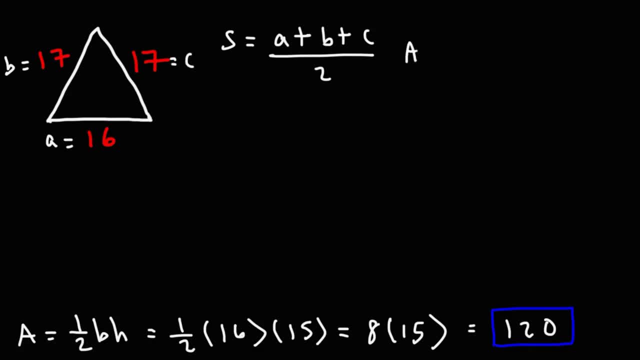 And c is 17. Now, once you have s, you can calculate the area using this formula. 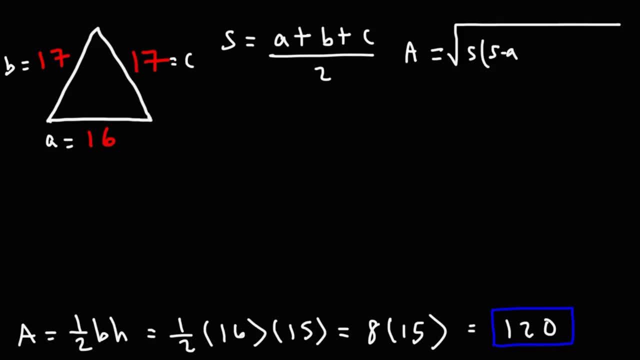 It's the square root of s times s minus a times s minus b times s minus c. So, what we're going to do is we're going to use this formula, or these two formulas rather, to confirm our answer to make sure that this answer is correct. 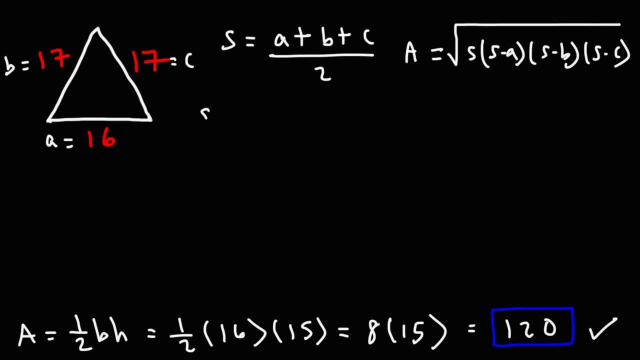 So, let's plug in the three side lengths into the first equation. So, it's going to be 16 plus 17 plus 17 divided by 2. 16 plus 17, that's 33. And 33, well, let's do it this way. 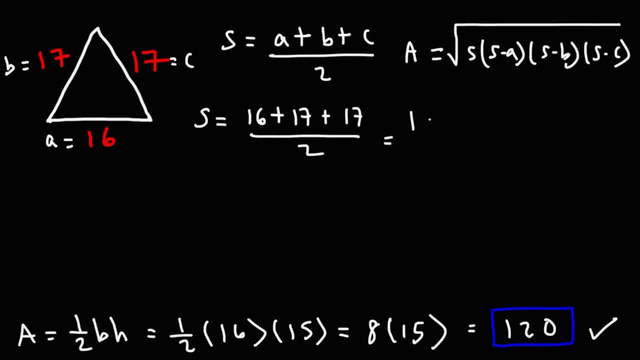 Let's add 17 plus 17 first. 17 plus 17 is 34. 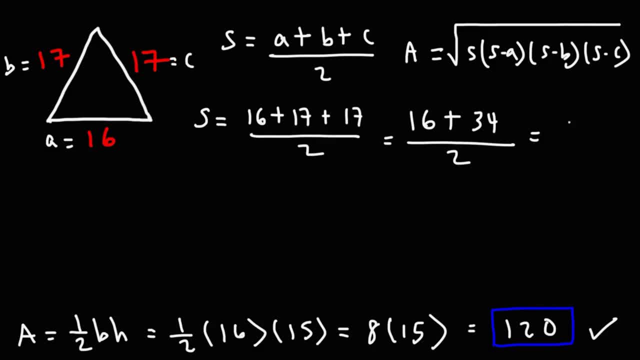 And 16 plus 34 is 50. Half of 50. It's 25. 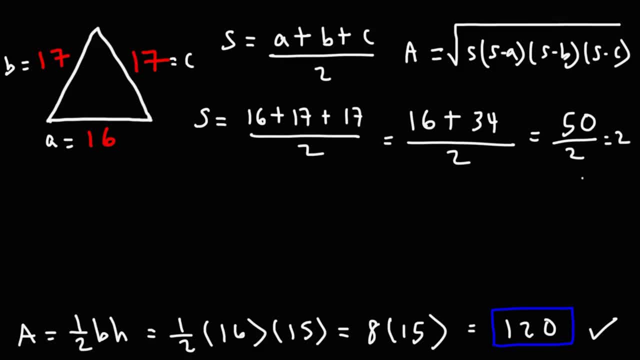 So, our s value is 25. 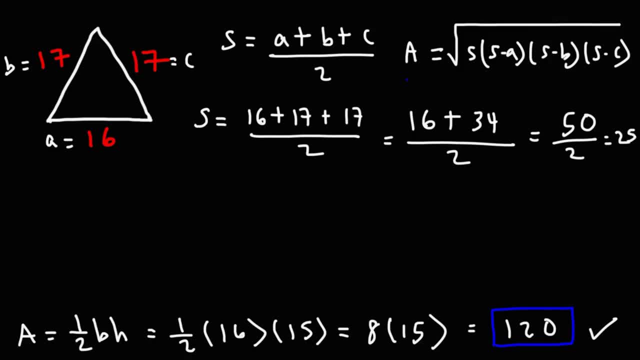 Now that we know the value of s, we can use this formula to get the area. So, we have the square root of 25. And then it's 25 minus a. 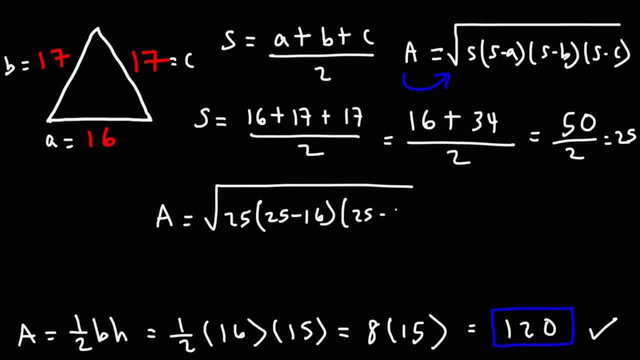 a is 16. 25 minus b. 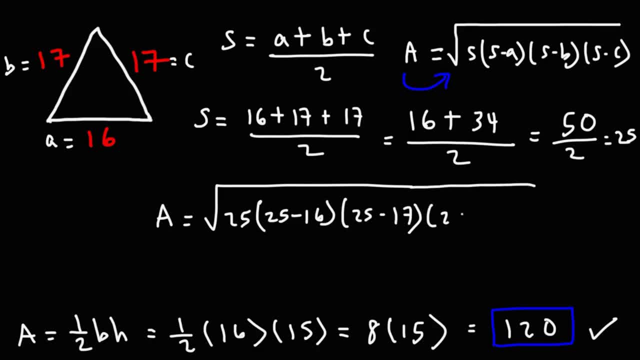 b. We know b is 17, and so is c. 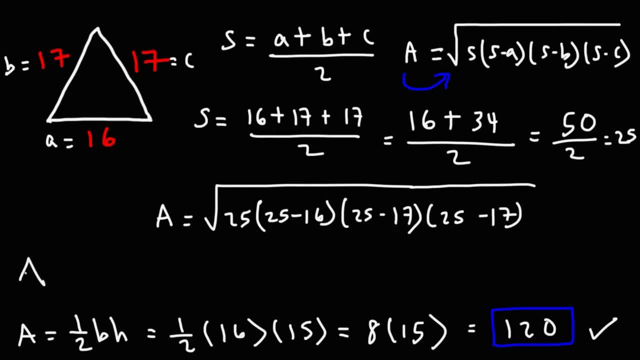 Now, 25 minus 16, that's going to be 9. 25 minus 17 is 8. And we have two of them. 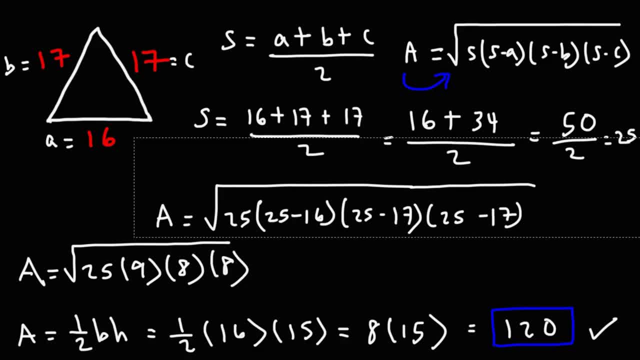 So, now let's do some simplifying. 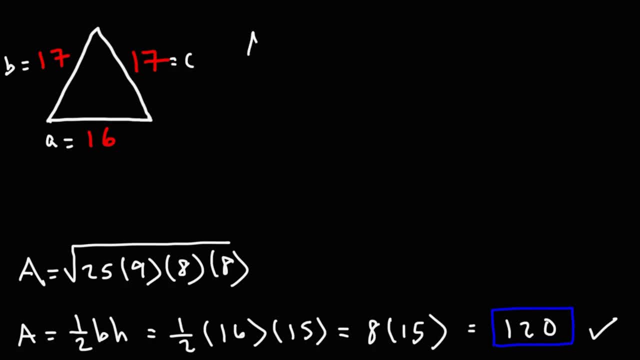 Now, I'm going to break this into three parts. 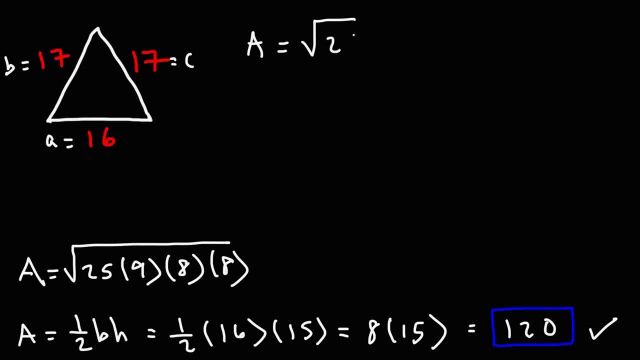 First, we have 25, which is a perfect square. So, I'm going to leave it by itself in a radical. 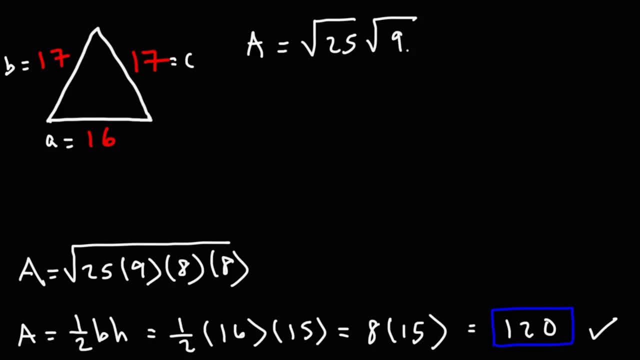 Then we have the square root of 9. Now, we can't take the square root of 8, but 64 we can. 8 times 8 is 64. 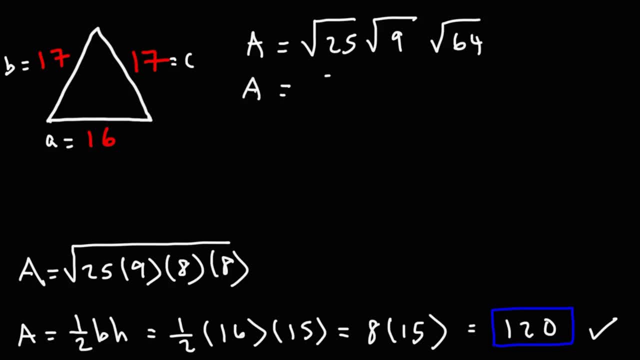 So, this is what we now have. The square root of 25 is 5. The square root of 9 is 3. And the square root of 64 is 8. 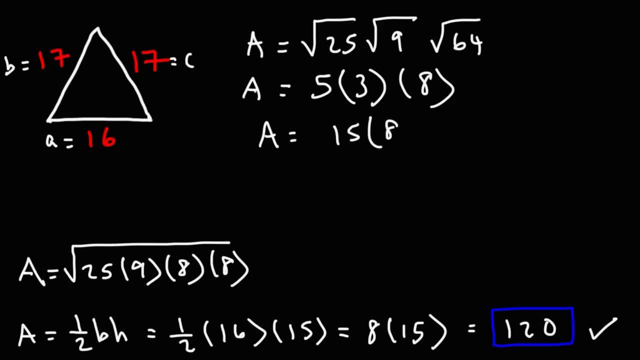 Now, 5 times 3 is 15. And we already know what 15 times 8 is. It's the same as 8 times 15, which is 120. 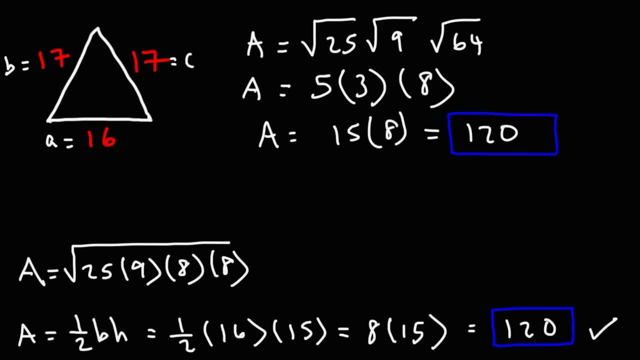 So, we do get the same answer, regardless of the methods that we choose to use. So, the area of this particular isosceles triangle is 120 square units. 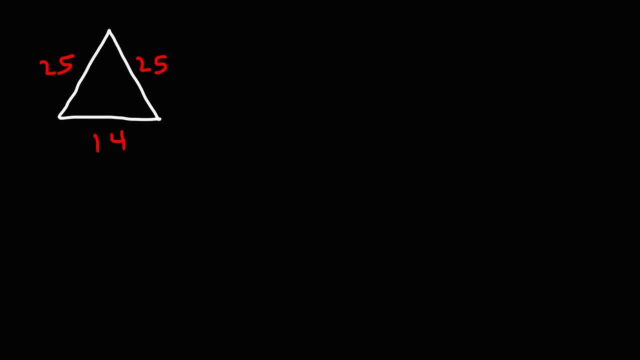 Now, for the sake of practice, go ahead and try this problem. Calculate the area of this isosceles triangle. Feel free to pause the video and work on this example. So, we're going to use the first method because it's a lot faster. 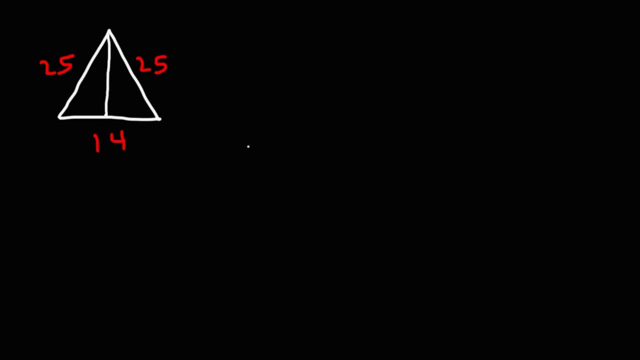 So, let's draw half of this triangle. And let's calculate the height. 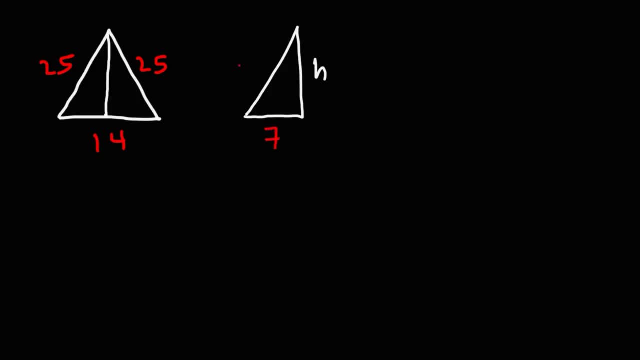 So, the base is going to be half of what it was, which is 7. But the hypotenuse is 2. So, it's still going to be 25. 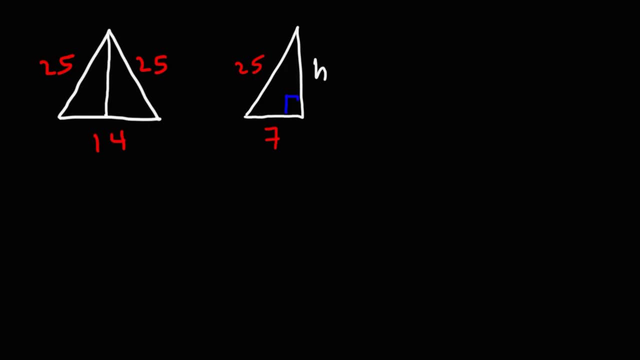 Now, at this point, it helps to know the special right triangles. For instance, there's the 3, 4, 5 right triangle. There's the 5, 12, 13 right triangle. There's the 8, 15, 17 triangle. 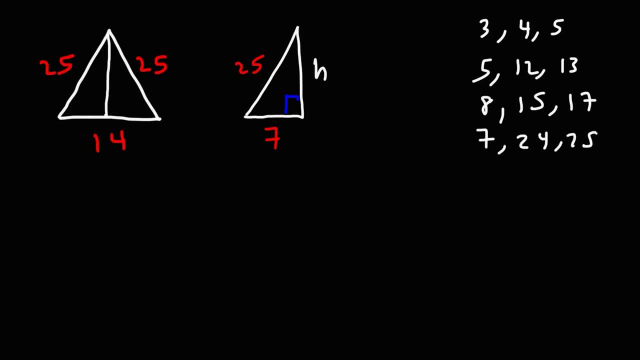 And then there's the 7, 24, 25 triangle, which is what we have. So, knowing this, you can automatically know that 8 is 24. Now, there's some other ones. 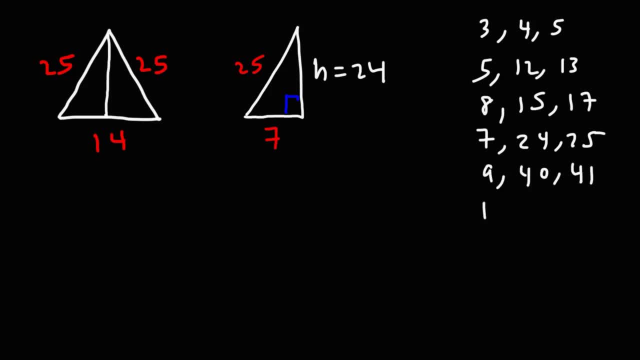 Like, 8 is 24. Like, the 9, 40, 41. And I believe 11, 60, 61. 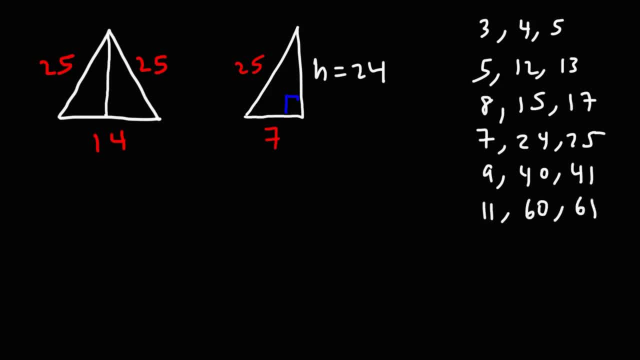 Let me make sure that's correct. 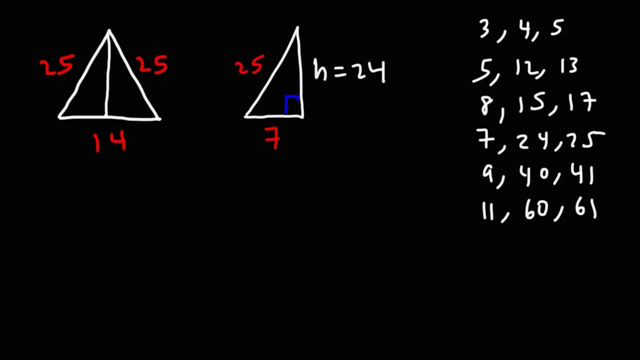 And it is. For the most part, you'll have one of those six variants or any multiple of them. 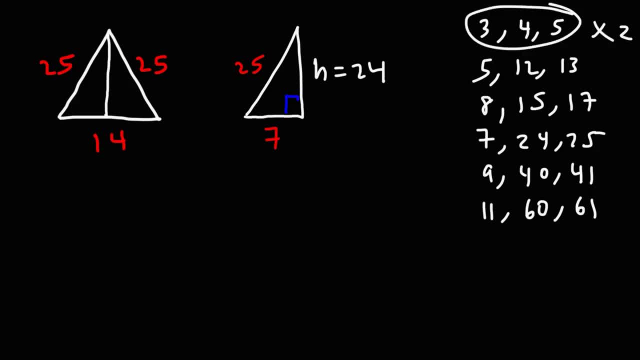 So, for instance, if you multiply this by 2, you can have the 6, 8, 10 triangle. Or if you multiply it by 3. The 9, 12, 15 triangle. So, any multiples of those numbers will work as well. 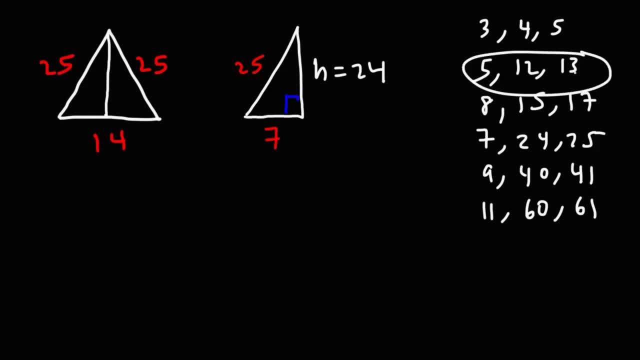 So, like this one, if you multiply it by 2, you have the 10, 24, 26 triangle. 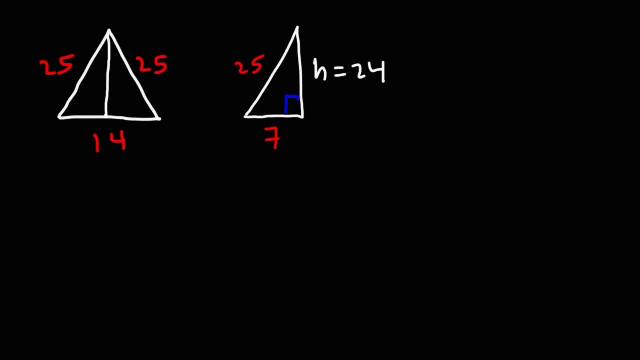 So, now that we know the height of the triangle, let's redraw the picture. So, the base is 14. And the height is 24. So, we can go ahead and use this formula. 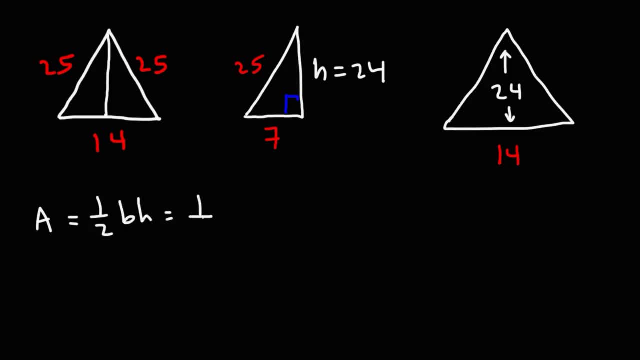 The area is going to be 1 half base times height. Base is 14. And the height is 24. 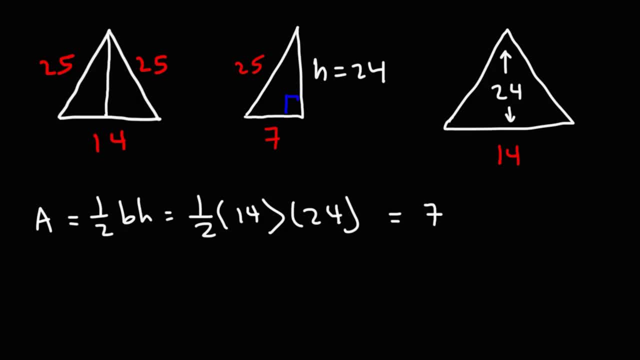 1 half of 14 is 7. And so, this becomes 7 times 24. 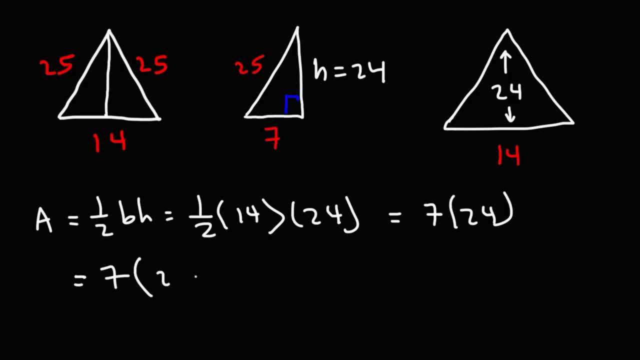 So, to do it mentally, let's break down 24 into 20 plus 4. 7 times 20. 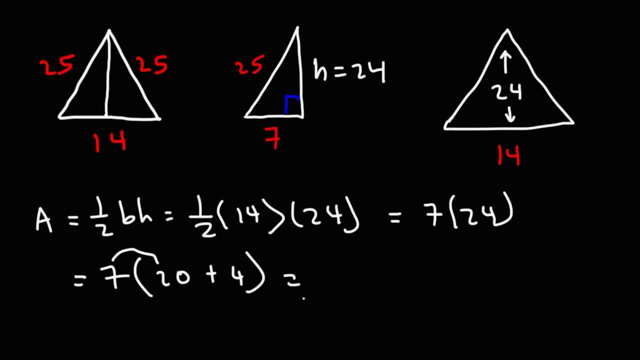 7 times 20. If you have 7 $20 bills, how much money do you have? That's going to be 140. 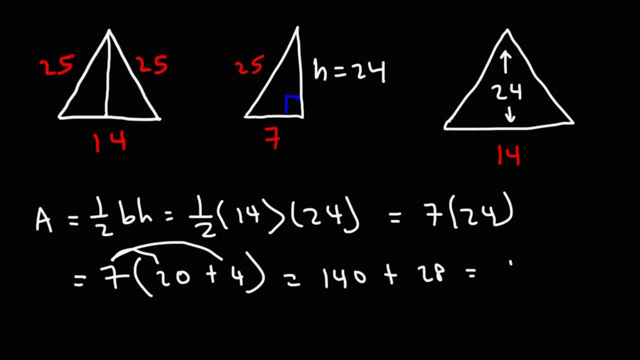 And then 7 times 4 is 28. Adding those two together, we get 168. 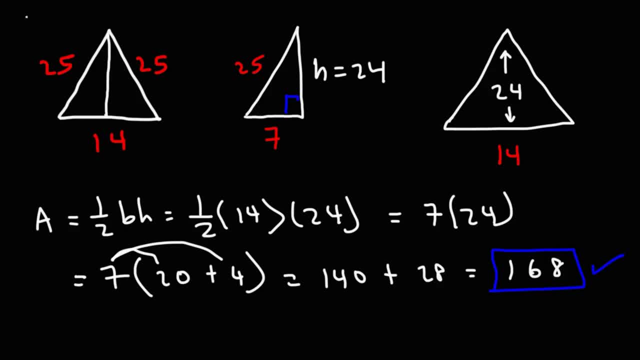 So, that's the area of the triangle. And let's confirm it real quick using Heron's formula. 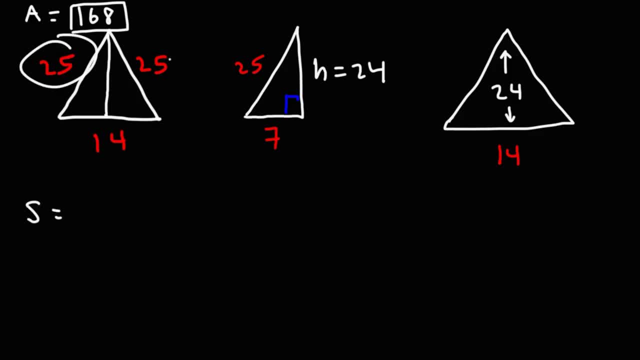 So, let's calculate S. S is going to be 1 half the sum of the three sides. So, 14 plus 25 plus 25 divided by 2. 25 plus 25 is 50. 50 plus 14 is 64. 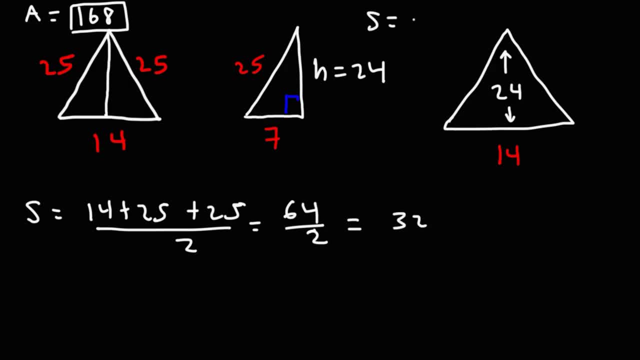 Half of 64 is 32. So, we can say S is 32. 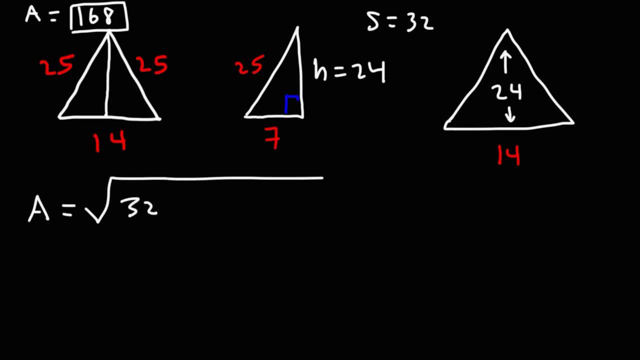 Now, the area is going to be the square root of S. And then S is going to be the square root of S. 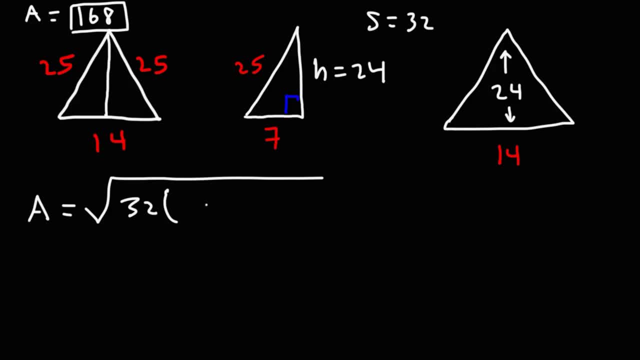 S minus A, let's say 32 minus 14, that's 18. And then S minus B, 32 minus 25, that's 7. 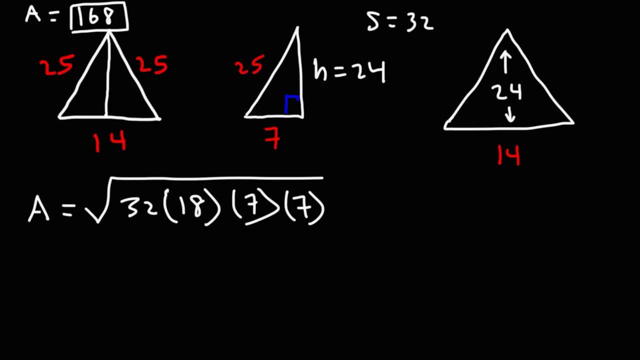 And then 32 minus the other 25 is 7 as well. 32, we can write that as 16 times 2. 18, that's 2 times 9. And 7 times 7, I'm going to leave it as 49. I'm trying to collect all the perfect squares here. So, 6 times 7 is 49. 16 is the perfect square. 2 times 2 is 4. We have 9 and 49. The square root of 16 is 4. The square root of 4 is 2. The square root of 9 is 3. 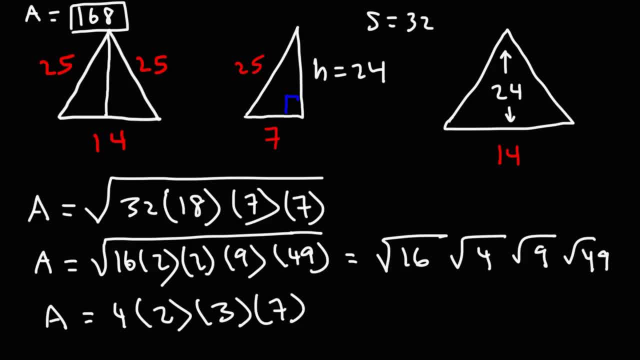 And the square root of 49 is 7. So, 4 times 2 is 8. And then 8 times 3 is 7. 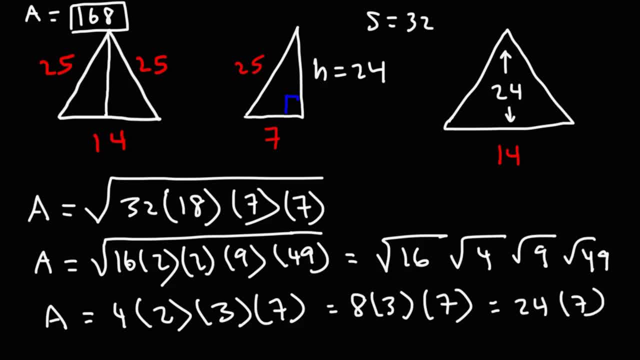 I mean, no, 8 times 3 is 24. But 24 times 7, that's going to give us the same answer of 168. So, we know we have the right answer. 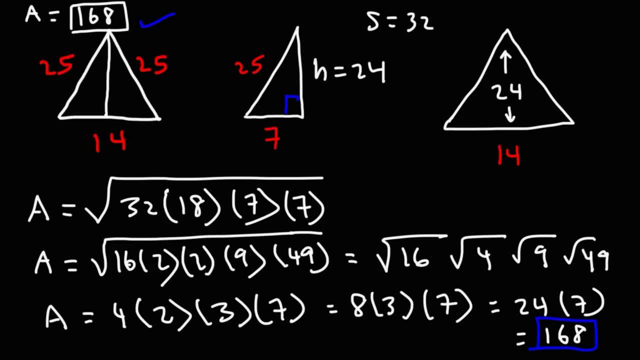 So, that's it for this video. Now you know two methods that you can employ in order to calculate the area of an isosceles triangle. 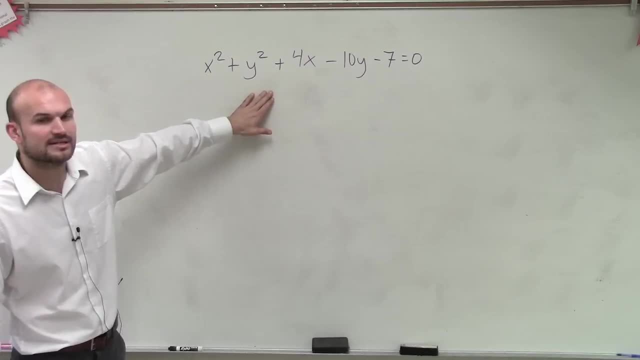 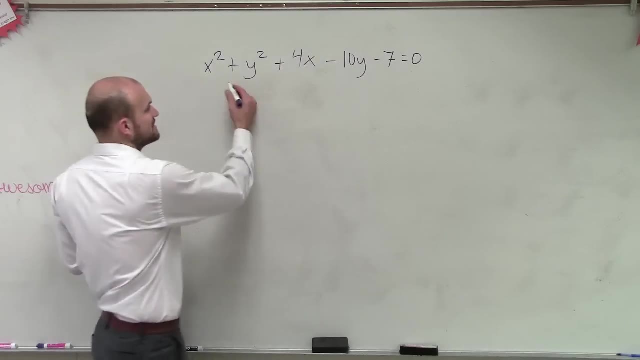 have to do for this problem is what we're going to simply do is we need to first be able to determine if it's in our standard form of our equation of a circle. So remember, standard form of equation of a circle looked like this: x minus, h squared plus y minus.